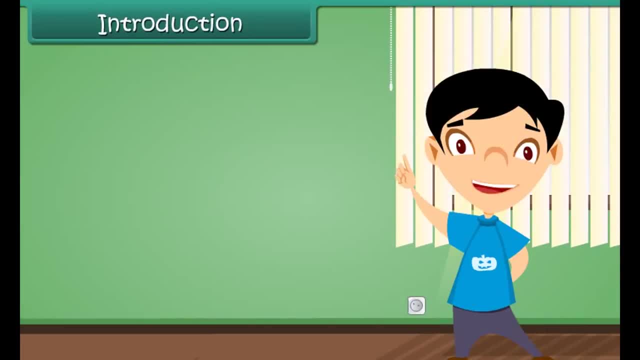 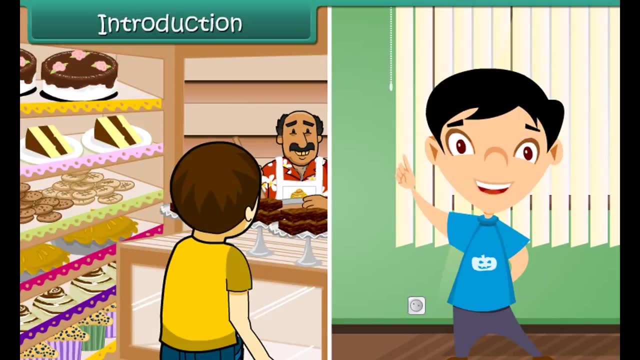 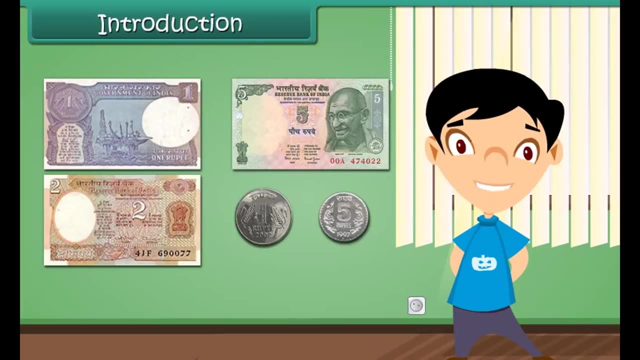 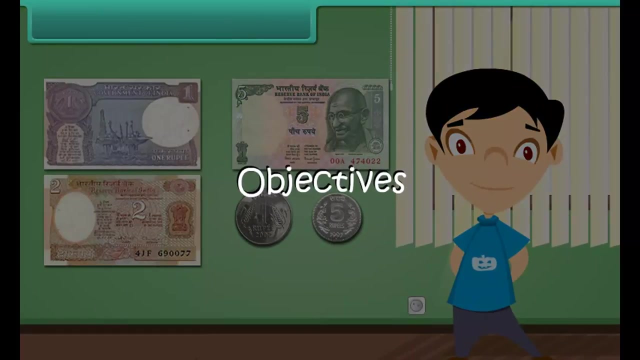 introduction: hello everybody. my name is Krish. I want to buy some chocolates. for this, I need to give money to the shopkeeper. without money, he will not give us anything. do you know what money is? okay, I will tell you more about money objectives at the end of this lesson. you'll 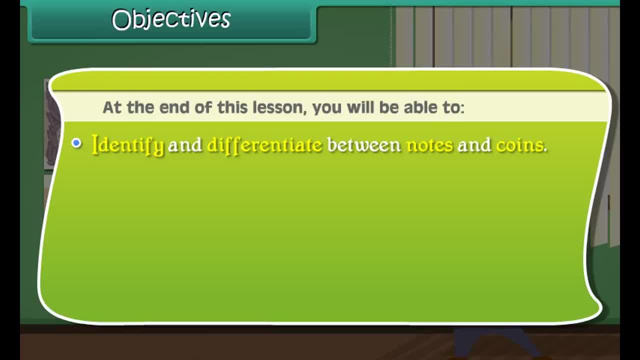 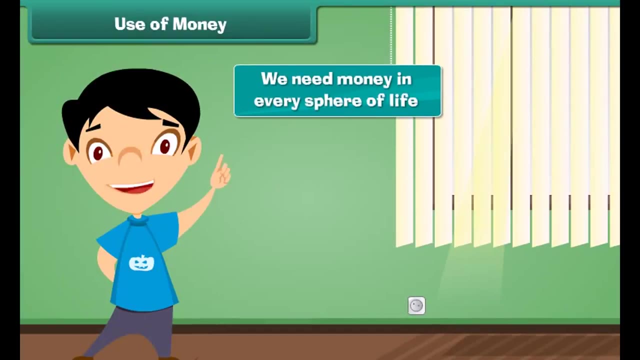 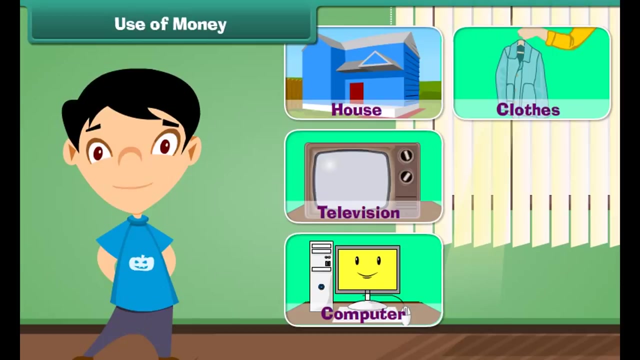 be able to identify and differentiate between notes and coins. make different combination of 20 and 50 rupees. note. know about saving, add and subtract money. understand correct combinations of notes and coins. we need money in every sphere of life. we require money to buy house television. 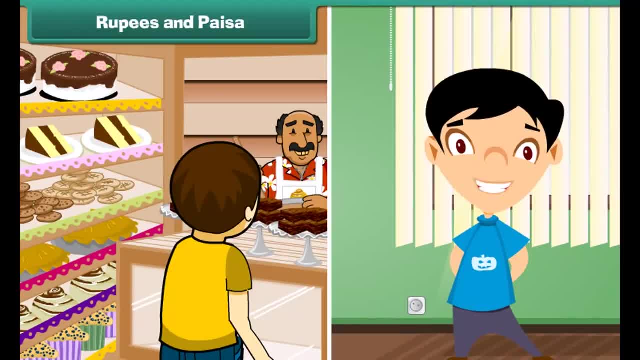 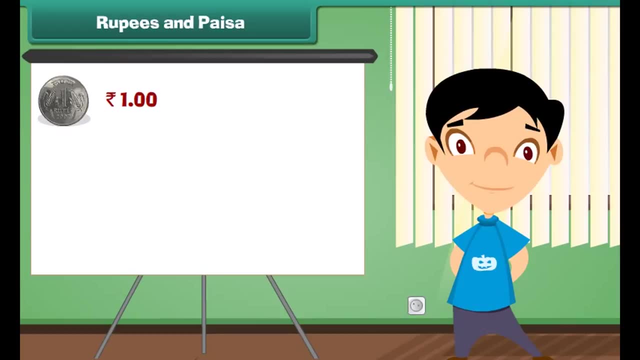 computer, Clothes, Grocery Stationery and many more things. When we go to market sometimes shopkeeper tells the amount in rupees and paise both. Let me show the correct way to write the price told by a shopkeeper. One rupee is written as rupee one. 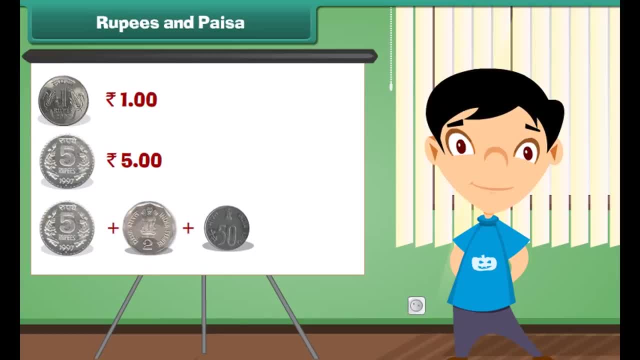 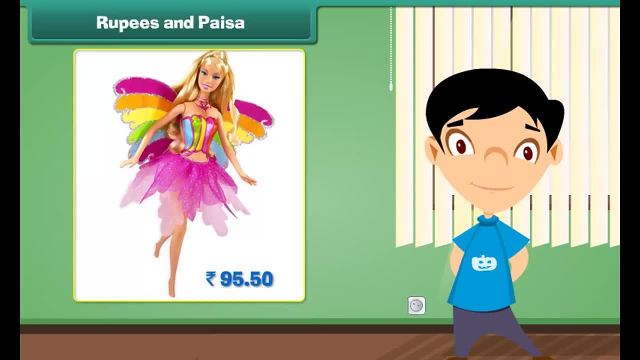 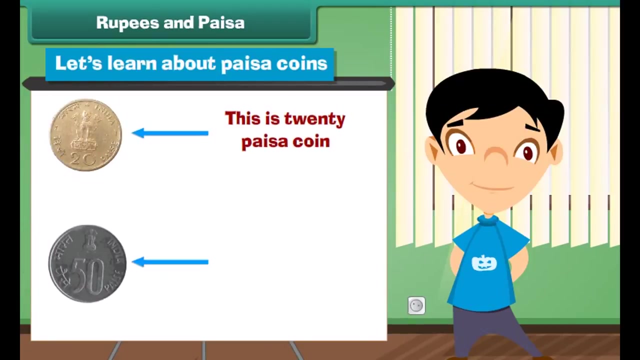 Five rupees is written as rupees five. Seven rupees and fifty paise is written as rupees seven point five zero. Look at this Barbie doll. Price is written on its label. We read the price as ninety five rupees and fifty paise. 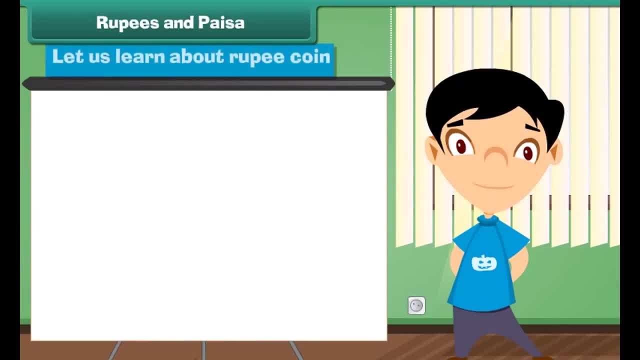 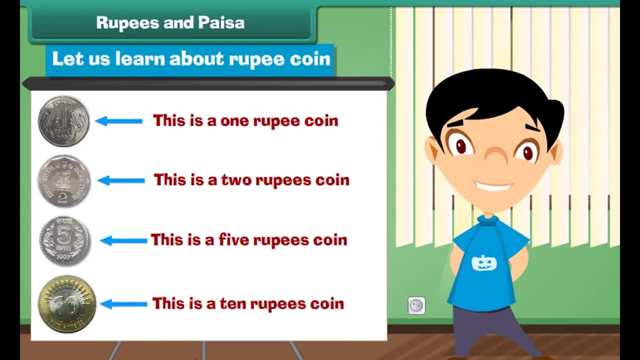 Let's learn about paise coins. This is twenty paise coin. This is fifty paise coin. Let us learn about rupee coin. This is a one rupee coin. This is a two rupees coin. This is a five rupees coin. 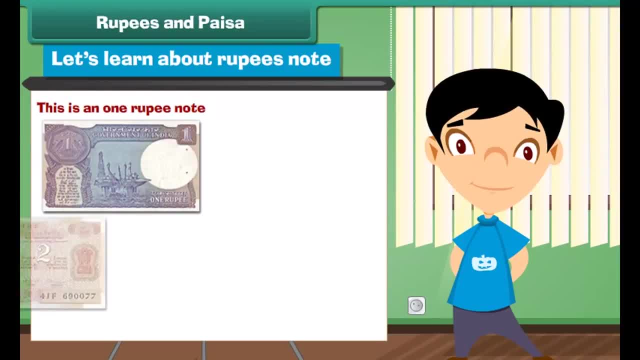 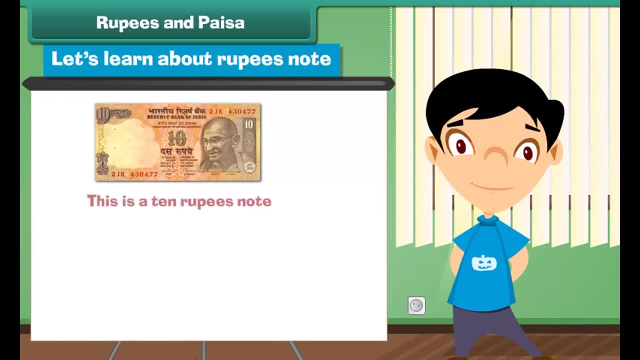 This is a ten rupees coin. Let's learn about rupees note. This is an one rupee note. This is a two rupees note. This is a five rupees note. This is a ten rupees note. This is a twenty rupees note. 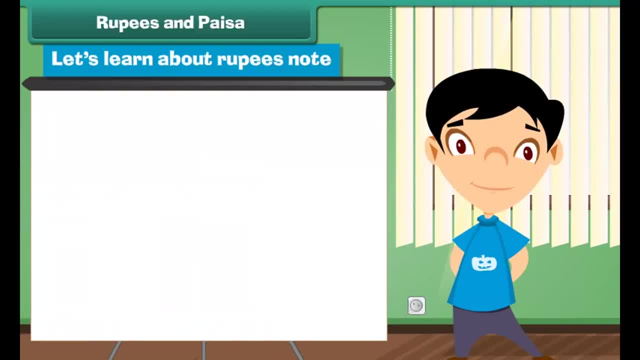 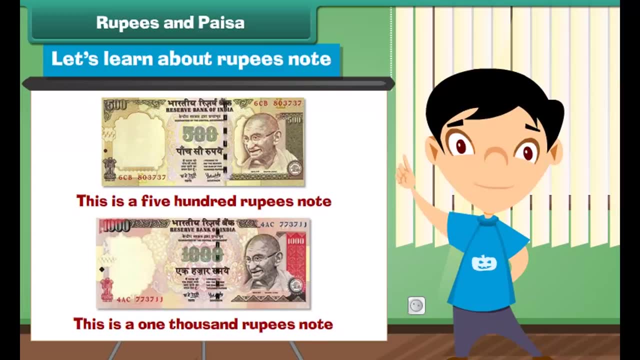 This is a twenty rupees note, This is a fifty rupees note, This is a hundred rupees note, This is a five hundred rupees note, This is a five hundred rupees note And this is a one thousand rupees note. 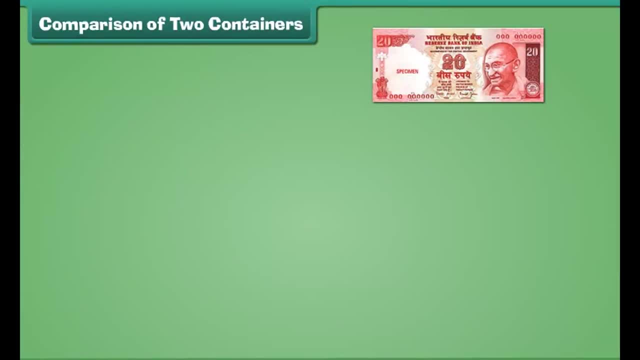 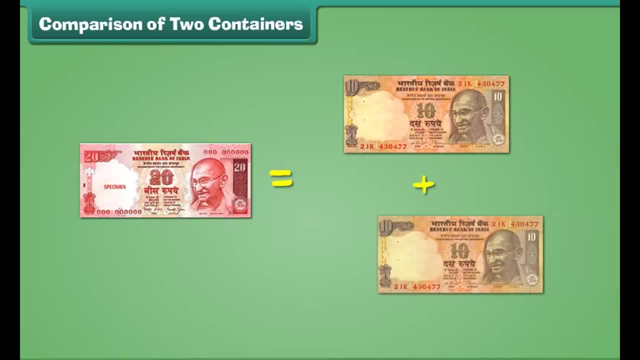 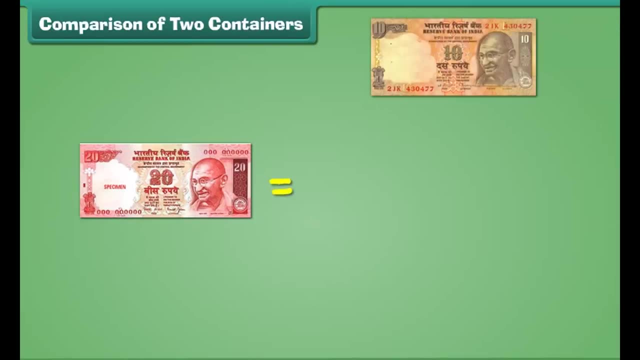 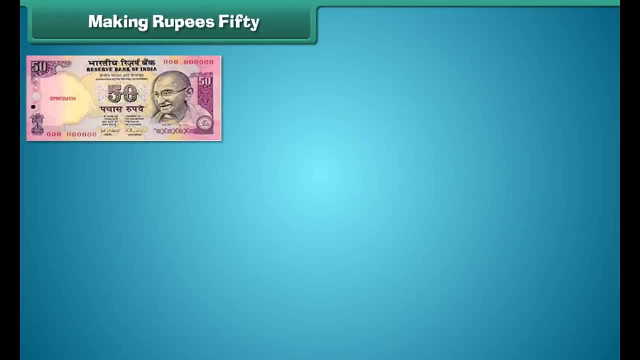 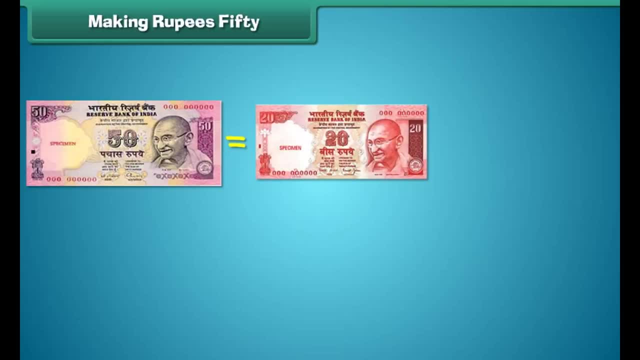 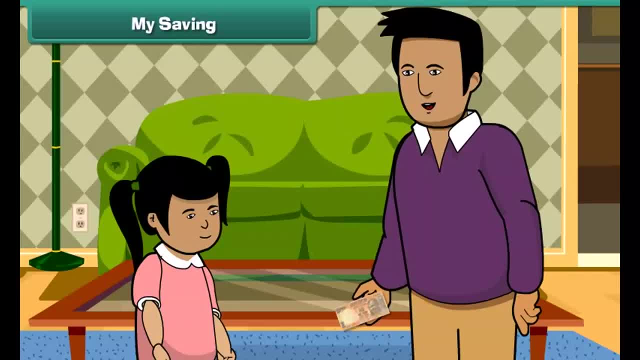 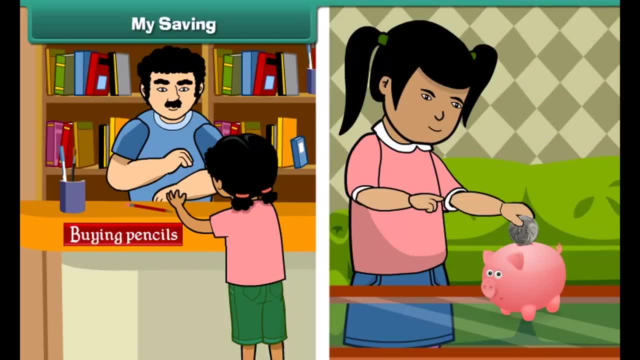 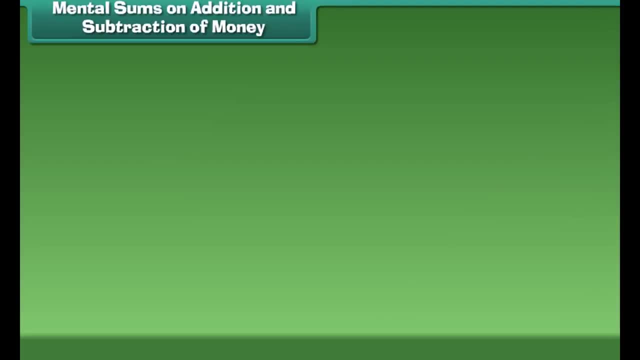 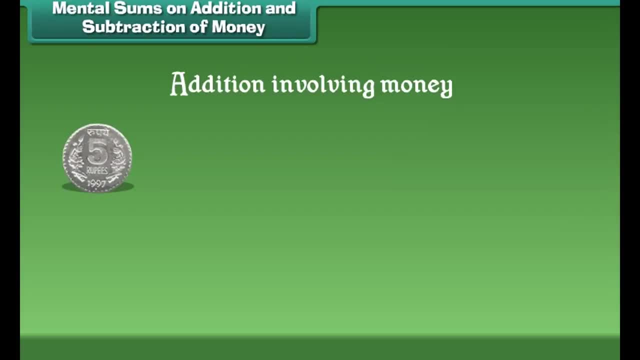 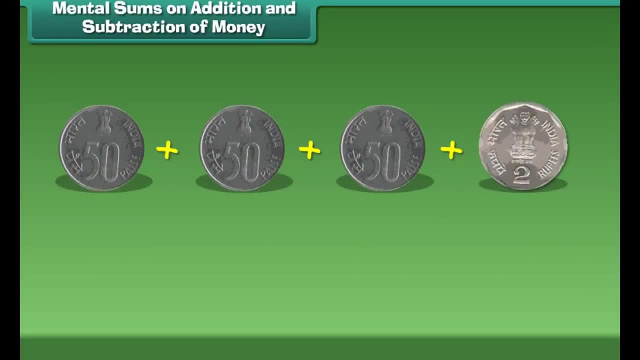 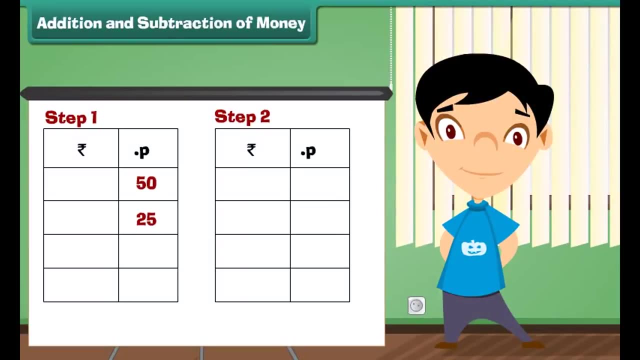 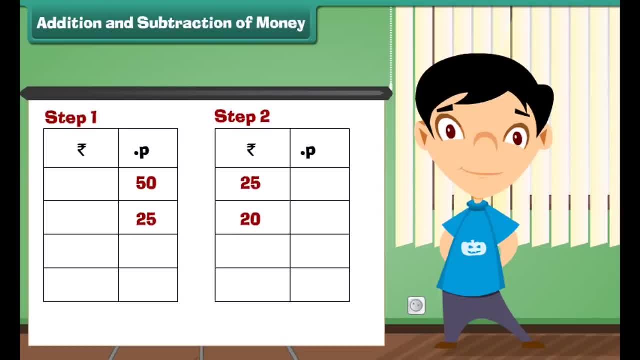 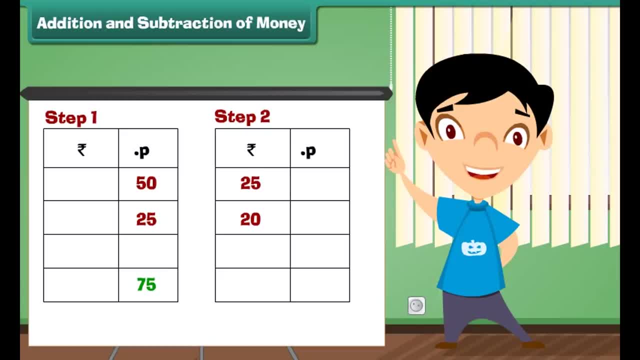 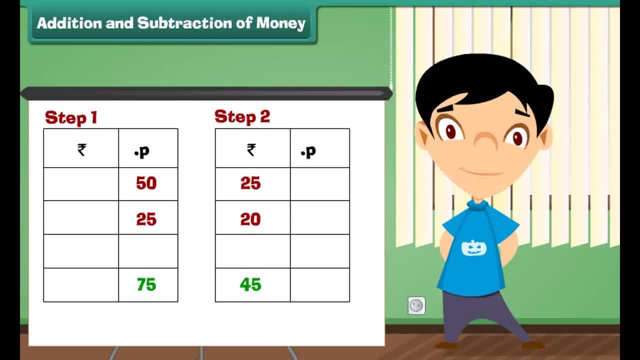 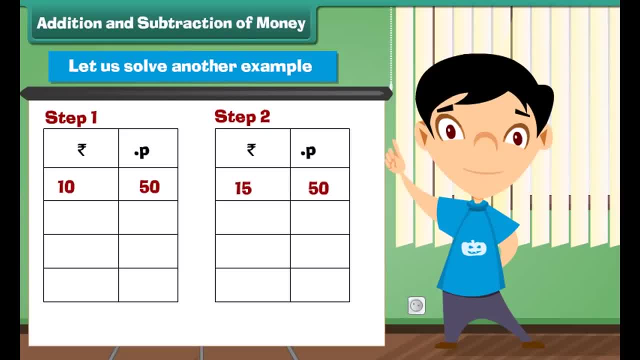 25 plus 20 is equal to rupees 45. Write 45 under the rupees column. Let us solve another example. What is the sum of 10 rupees 50 paisa and 15 rupees 50 paisa? Step 1: 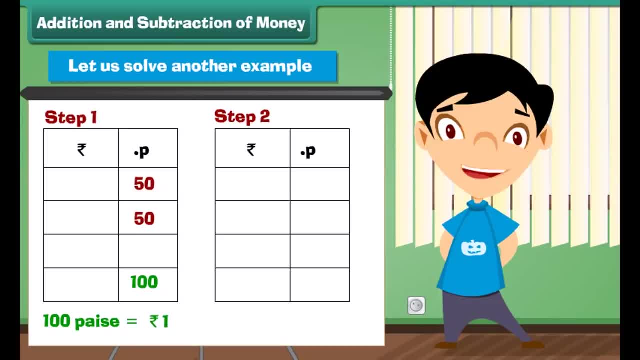 Write the numbers in correct column. Step 2: Add the numbers in paisa column. 50 plus 50 equals 100 paisa, But we know that 100 paisa is equal to 1 rupee, So we write two zeros below the paisa column. 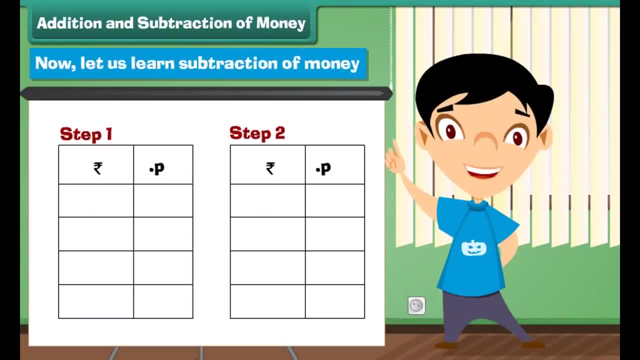 And take 1 as carry. Step 2: Add the numbers in rupees column. 1 plus 10 plus 15 equals 50 plus 50 is equal to rupees 26. Write 26 under the rupees column. Now let us learn subtraction of money. 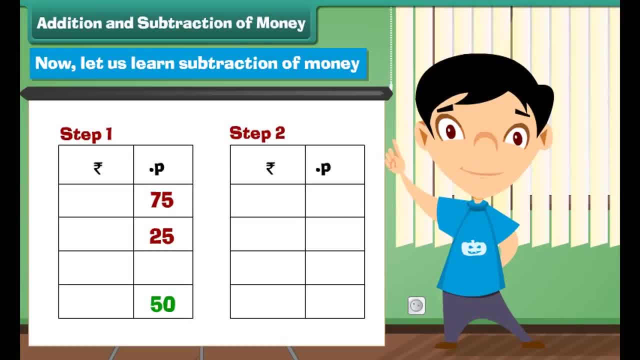 Subtract 10 rupees: 50 paisa from 40 rupees and 75 paisa. Step 1: Subtract the numbers in the paisa column 75 minus 25 is equal to 50 paisa. Write 50 under paisa column Step 3. 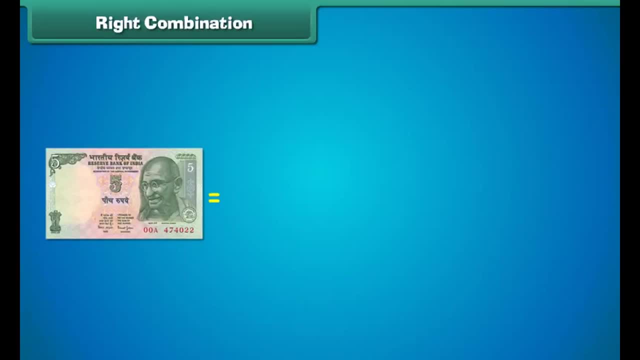 Subtract the numbers in the rupees column 40 minus 10 equals 30. Tip 10: Write 30 under rupees column. Lets learn about some right combinations of notes and coins. 1 five rupee note is 5 100 rupees coins. And then we have a matchadas بين 50 000 and 500 000 rupees maats and 5 1000 rupees coins.